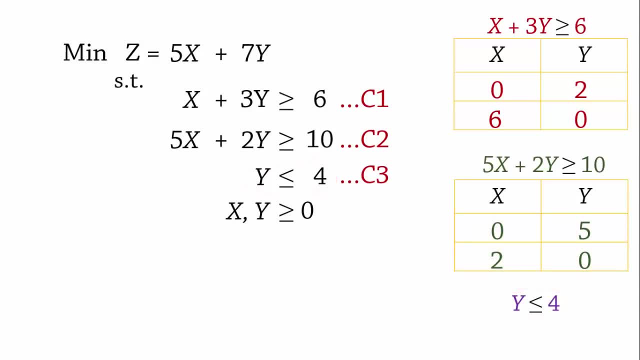 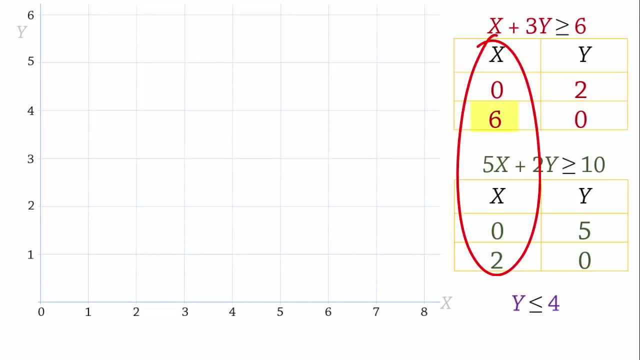 For constraint 3, y is just always less than or equal to 4, irrespective of the value of x. In drawing the graph, note here that the highest value of x is 6 and the highest value of y is 5.. And that is what tells us how far we need to go on the x and y axis. 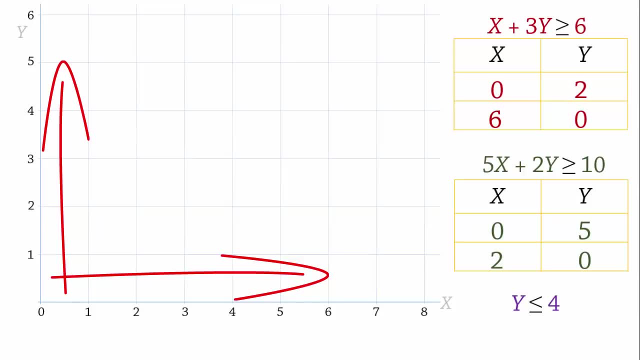 You can see that I went a little bit higher than 6 on the x axis and a little bit higher than 5 on the y axis, because I have the space. So, drawing the line for the first constraint, we have the points 0,, 2, and 6, 0, which we 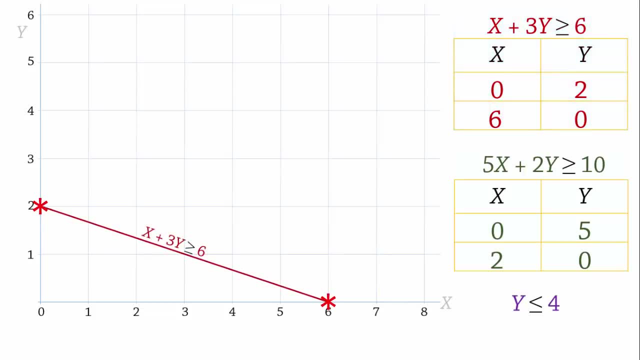 join to form the constraint line. For the second constraint. we have 0,, 5, and 2,, 0, which we also join to form the constraint line. For y less than or equal to 4, the line is simply at y equals 4.. 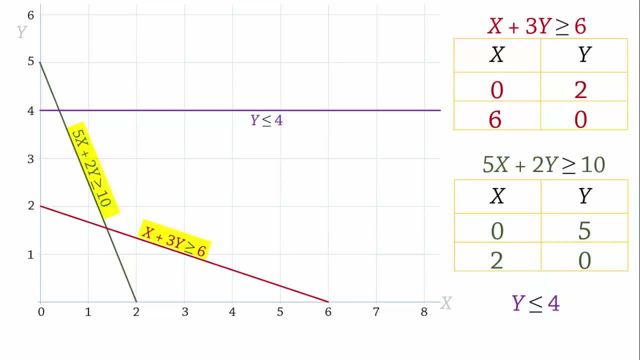 Now, since the first two constraints are greater than constraints, they will be satisfied in the region above the lines away from the origin. And y less than or equal to 4 is simply satisfied below the line. The direction of the arrows show that the region satisfying all the constraints at the 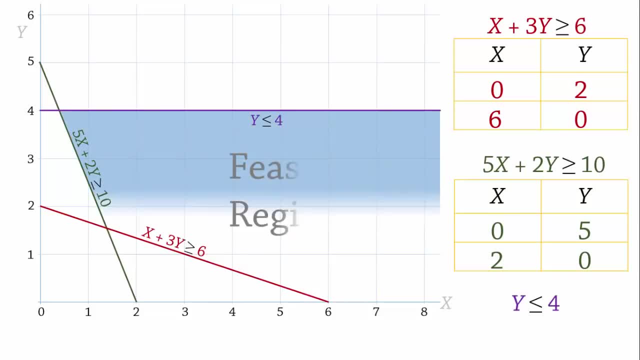 same time called the feasible region, is this area shaded in blue? Now, the optimal solution to this problem will occur at an extreme or corner point of this feasible region. Let's label them A, B and C for reference purposes. Now recall that the objective function is 0. 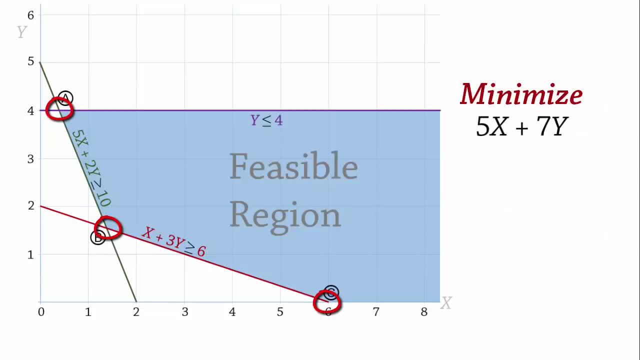 The objective function is to minimize 5x plus 7y. So the corner point that gives us the minimum value of the objective function is the optimal point. Instead of testing every single point, we will use the objective function line approach. We begin by setting the objective function to any number of our choice. 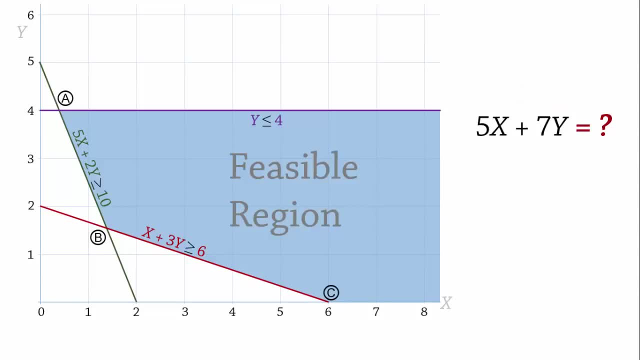 To make the process easy, we can simply multiply the coefficients of x and y. In this example, we have 5 times 7, which equals 35.. 35 seems to be appropriate. Note that if this number is too small or too large, you can always multiply or divide it. 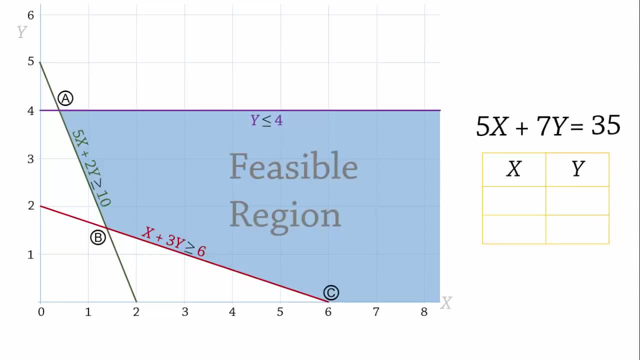 by an appropriate value. Next we find the points to draw the objective function line: When x equals 0,. y equals 5, and when y equals 0, x equals 7.. So the objective function line is this blue dotted line here.